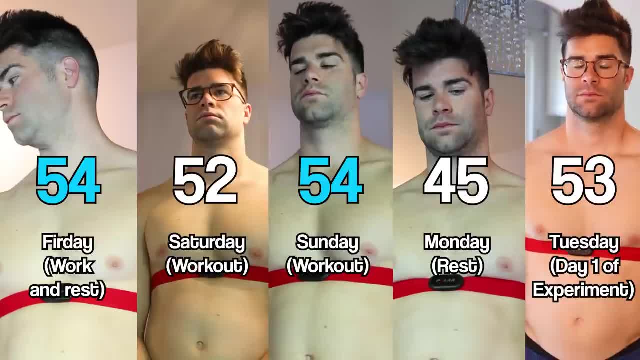 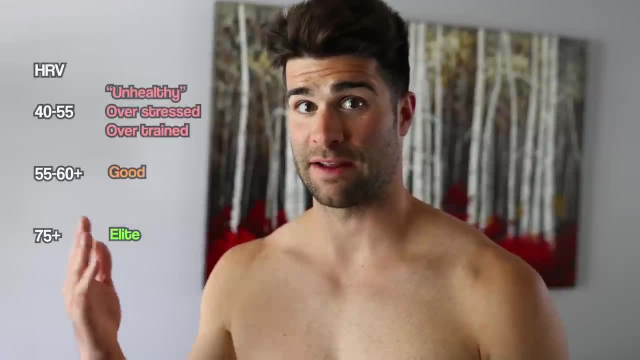 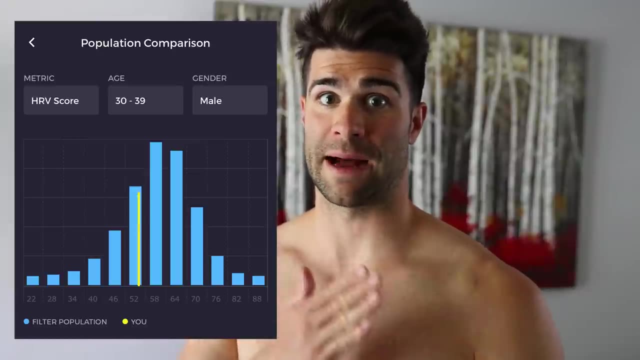 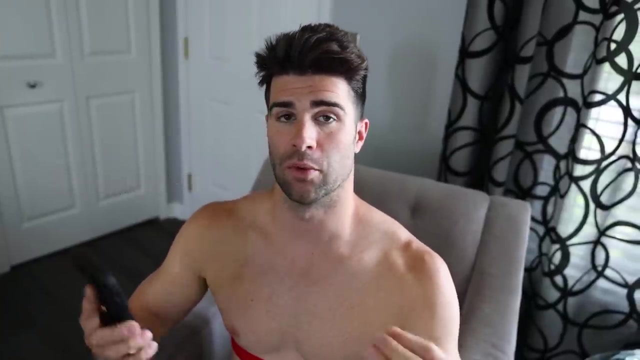 I was at a 45. All of my heart rate variability measurements, even my highest ones over the past five days, were all beneath the average for my age group. So apparently one of the quickest ways to immediately improve heart rate variability is doing breathing exercises, And one of the 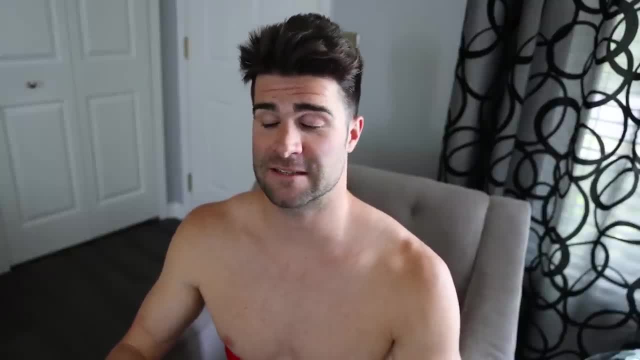 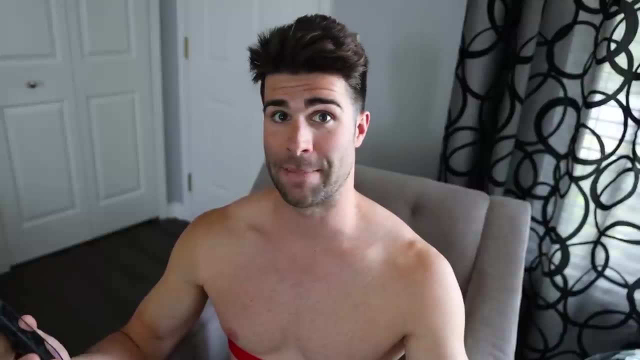 simplest breathing exercises to do for this instance is a five count inhale and a five count exhale. That's exactly what I'm going to try right now And I'm going to see if I get a better reading immediately. Looking closer at HRV, that variation between each heartbeat. 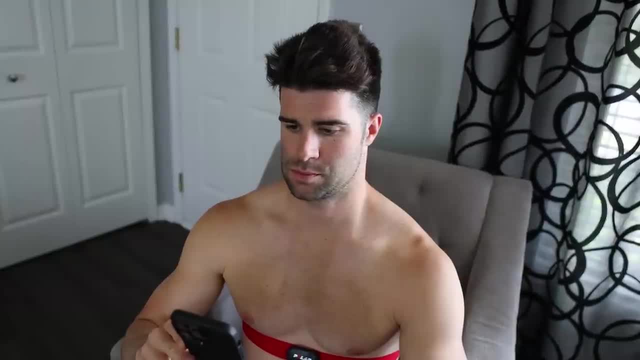 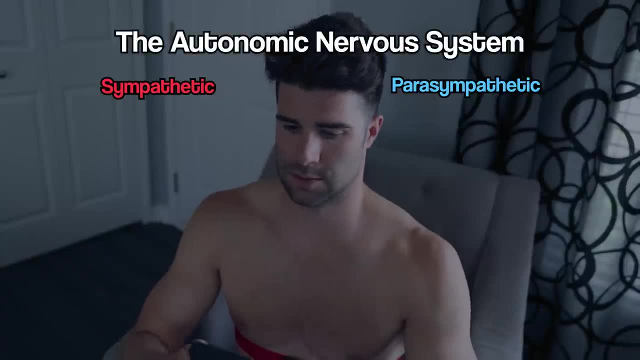 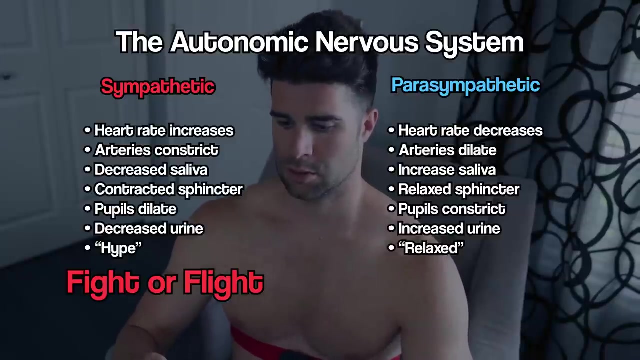 essentially indicates how responsive or balanced your nervous system is, between the sympathetic nervous system and parasympathetic nervous system, The main components of our autonomic nervous system which are responsible for controlling most of our body's involuntary functions, Whether that is going into fight or flight mode when needed to perform intensely. 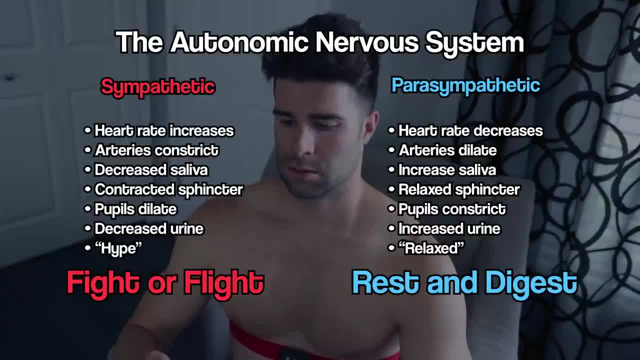 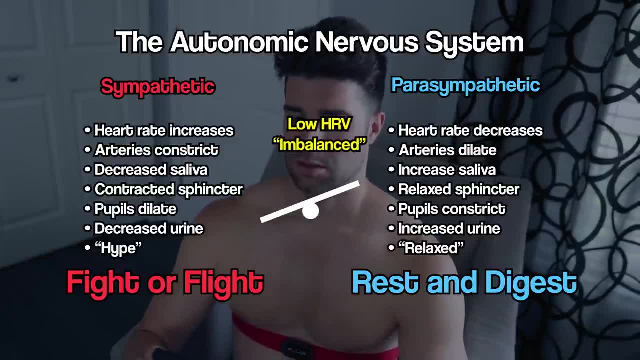 or going into rest and digest mode when needed to repair and recover. Now, a lower HRV score can indicate an imbalance between these two responses or an inability to switch between the two efficiently. Now, research has shown that this simple breathing technique consisting of 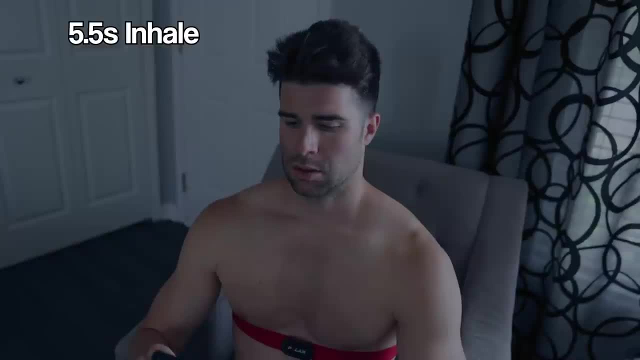 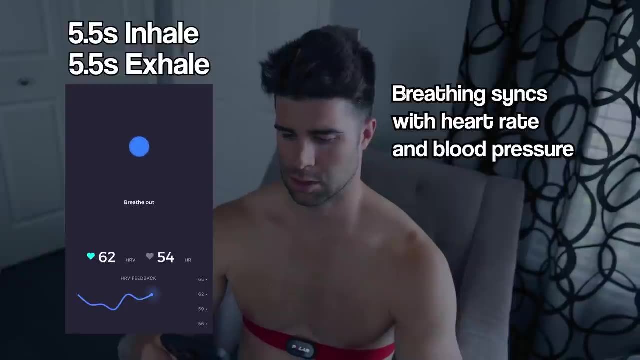 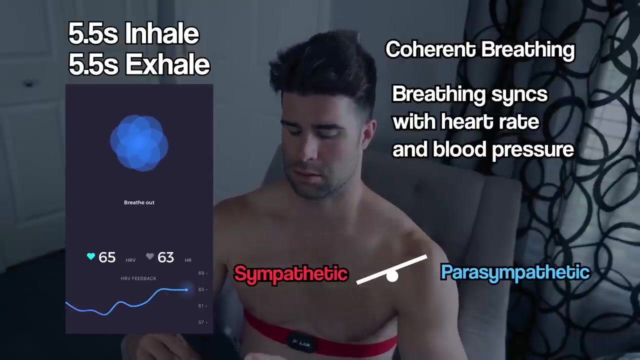 approximately a five and a half second inhale, followed by a five and a half second exhale, physiologically allows our breathing pattern to synchronize with our heartbeat in a state known as coherence. This, in return, allows our autonomous nervous system to become balanced and better. 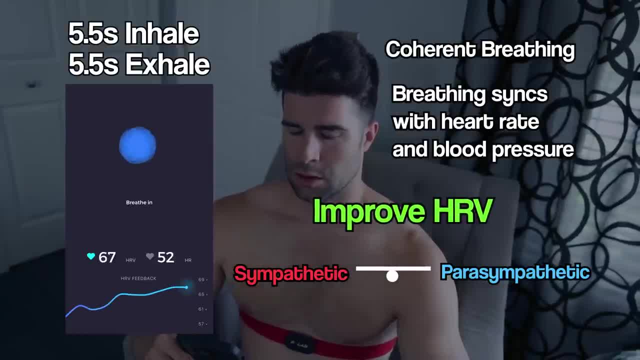 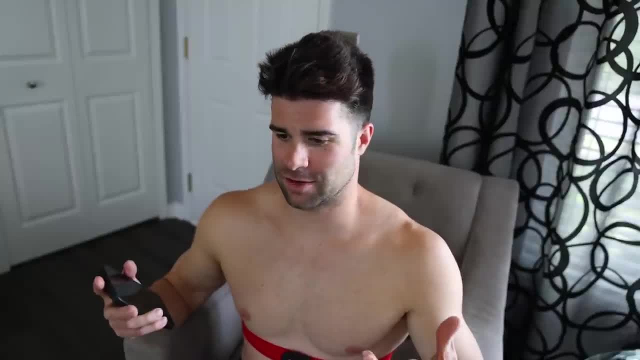 We're ready to respond, thus improving the HRV score. Would you look at that? All right? so that's very promising. In fact, I actually feel a lot more refreshed and clear right now, So I'm actually going to just get back to work for about an hour or two and then 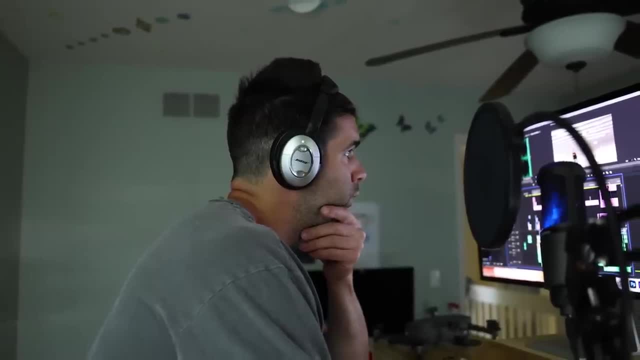 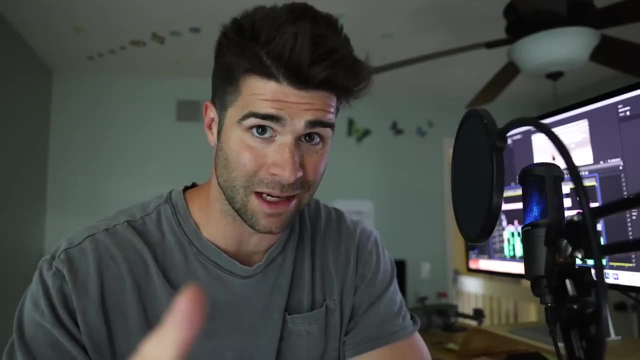 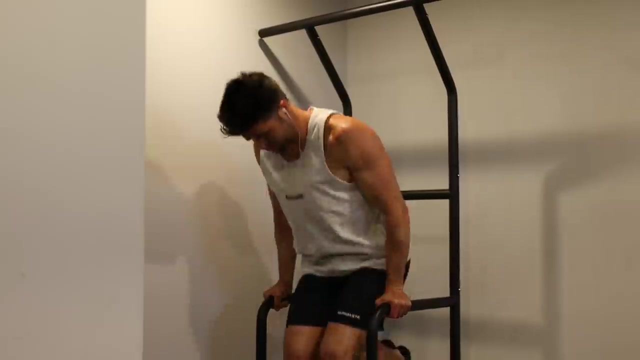 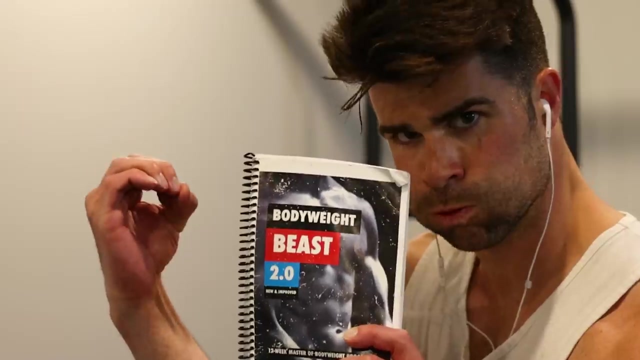 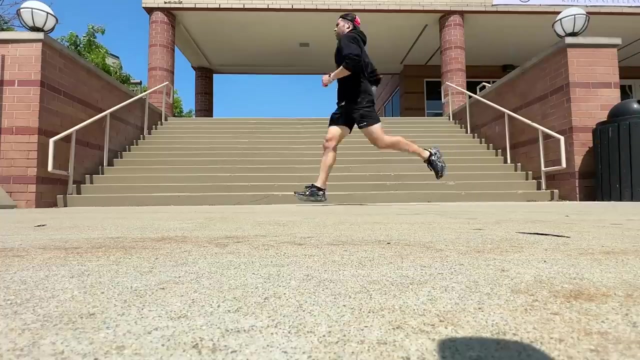 I'm going to get on with the rest of the day. That quick fix with a simple breathing routine left me feeling balanced and what I felt were some good benefits Done with work. for now I'm going to get in a workout, And I was quite pleasantly surprised at how smooth the workout went. I felt energized. 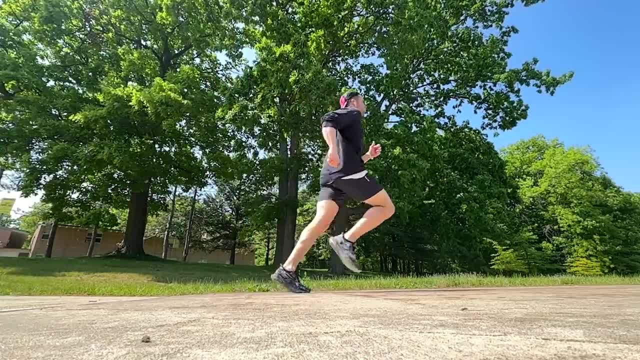 able to just dial in and perform. Could something as simple as a three minute breathing routine have that much positive impact on physical performance? Well, I was inspired. I was inspired. I was able to just dial in and perform. Could something as simple as a three minute breathing 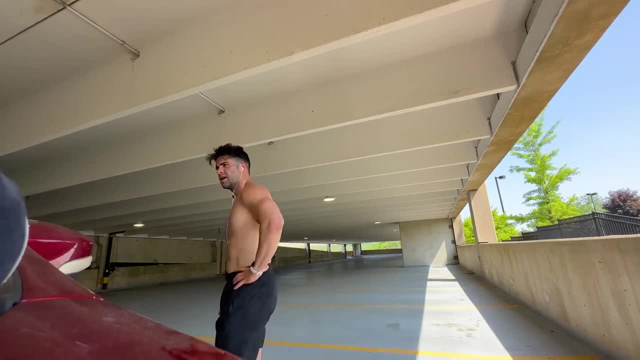 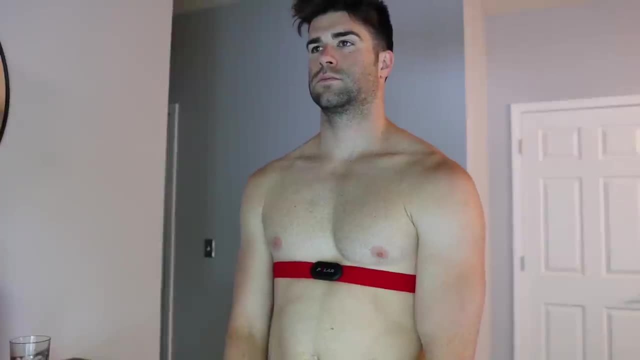 routine have that much positive impact on physical performance. Well, I was inspired. I was inspired to try more and find out more. By the way, great news guys, They fixed her. They fixed her While being able to improve my heart rate variability and become more balanced in the middle of the day led to some great benefits. I ultimately wanted to strive to have a more consistently high morning HRV result, But on day two, after not so great of a night's sleep, my morning HRV was once again not the best. So my HRV this morning is not the best. It is 53, so it's not much worse than it already was. But yeah, terrible sleep. I think if I would have got better sleep I probably would have had way better HRV today. Anyways, 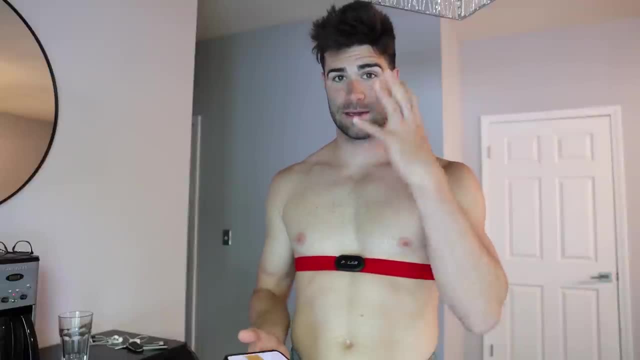 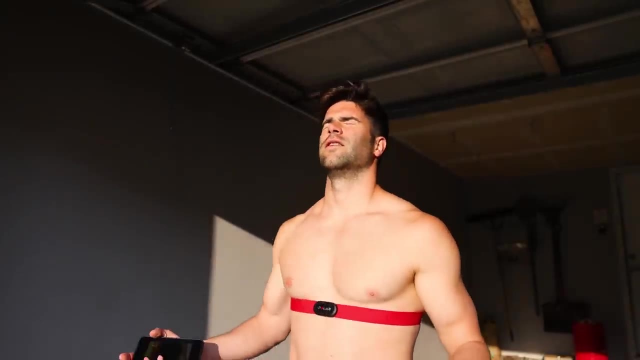 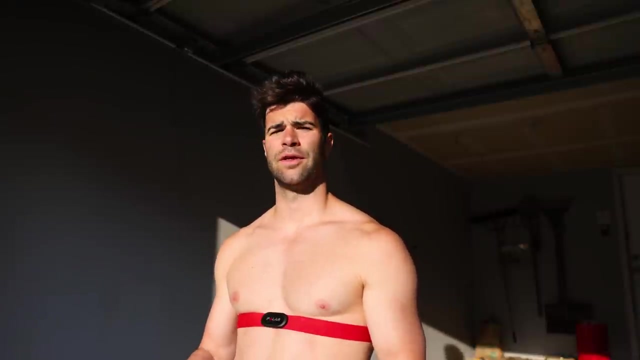 I'm going to go outside right now and get some sunlight immediately on the body, because there's a little biohack there. Ooh, look at that glow. Oh, So apparently getting exposed to ideally sunlight first thing in the morning is good for your circadian rhythm, as in it will help you go to sleep. 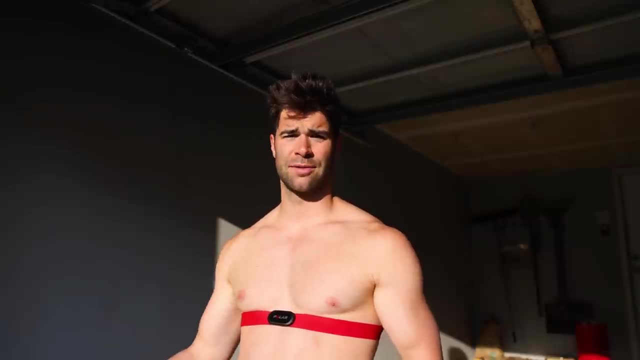 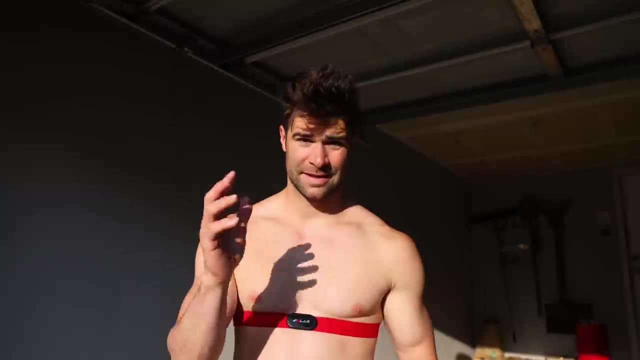 And if you're not getting exposed to it, you're going to go to sleep faster and stay asleep longer, And then therefore, getting more sleep would help increase your recovery and that would help increase your HRV. This is actually something I've been implementing over the past about 30 days. I was planning 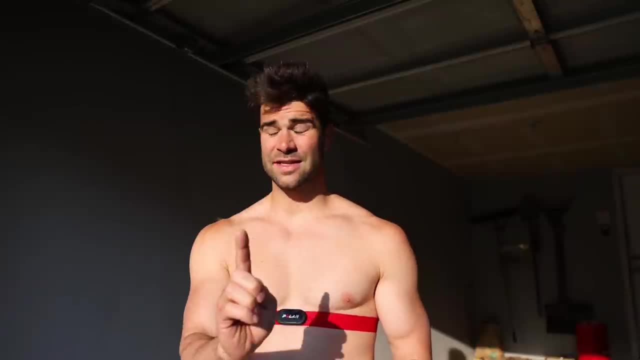 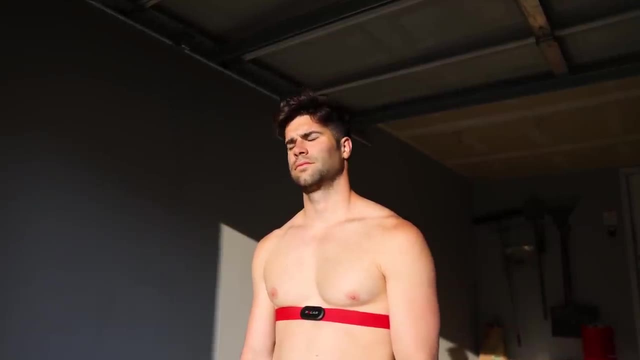 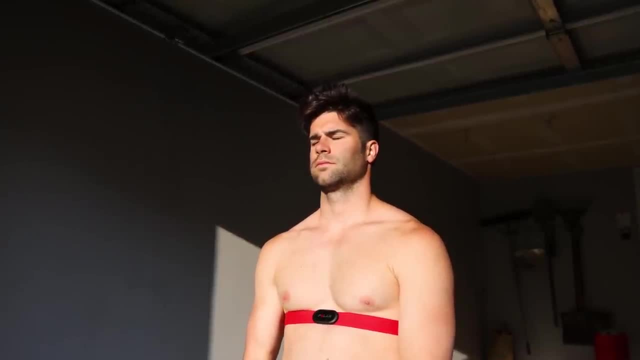 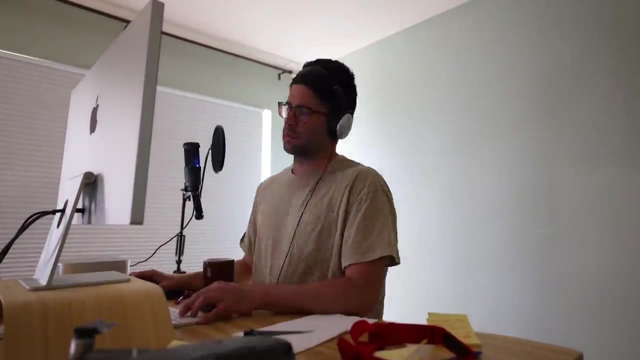 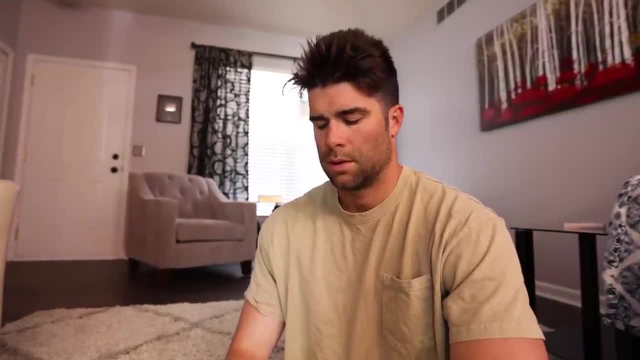 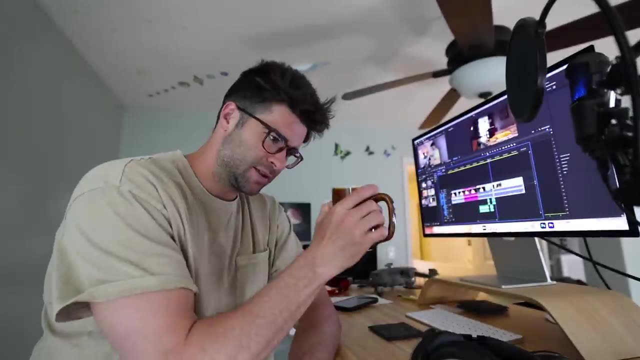 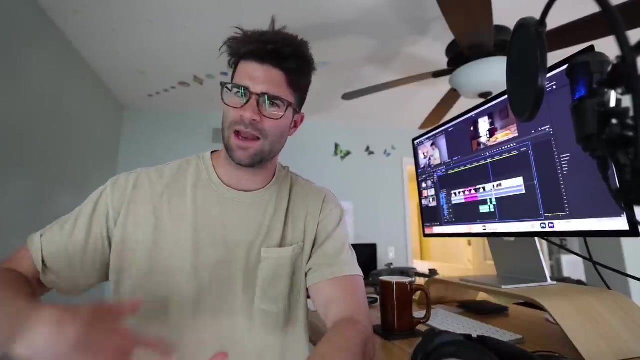 On top of this, there were a few more things I was going to try to do or not do this day that would hopefully positively affect my heart rate variability. I just finished my second cup of coffee and I think I'm going to cut it off here, because I've been noticing I've just been consuming more and more coffee. 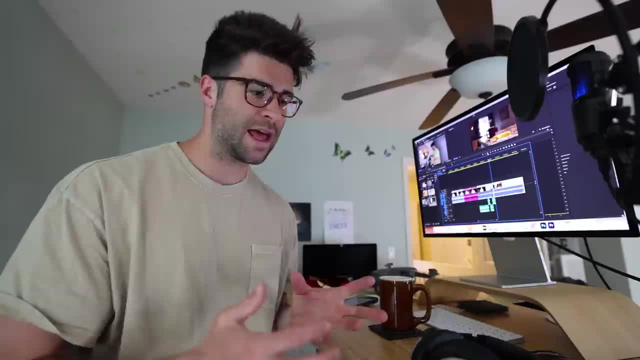 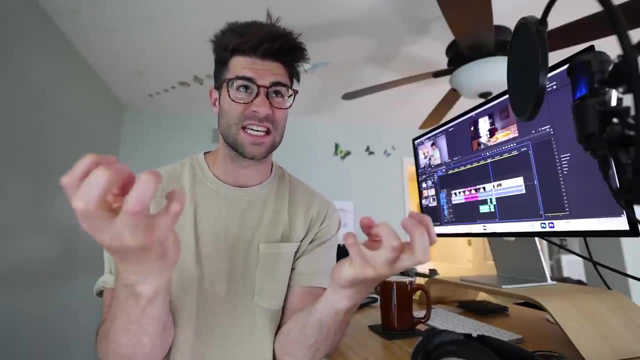 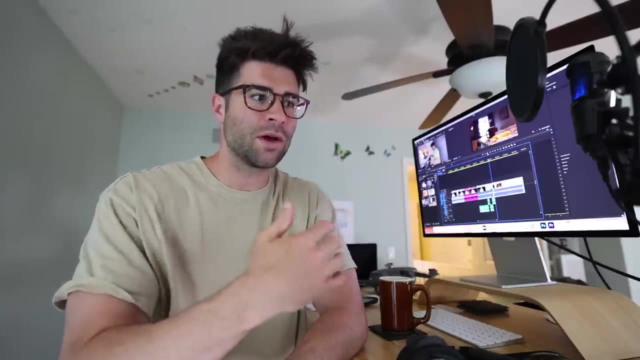 And I think consuming too much coffee or too much caffeine has been one of the reasons that's been leading me to getting trapped in this sympathetic or constantly agitated, stressed, just can't relax state. So, yes, temporary performance might decrease here today, but I'm hoping overall, hopefully slowly decrease. 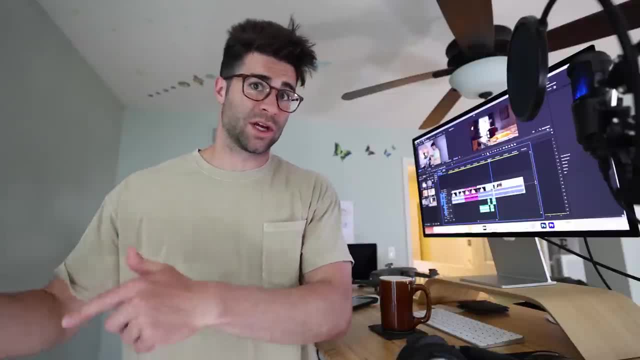 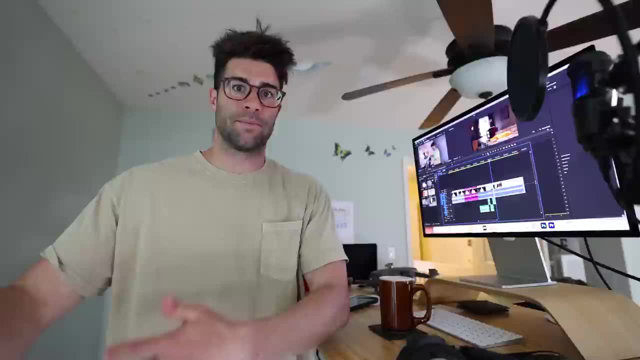 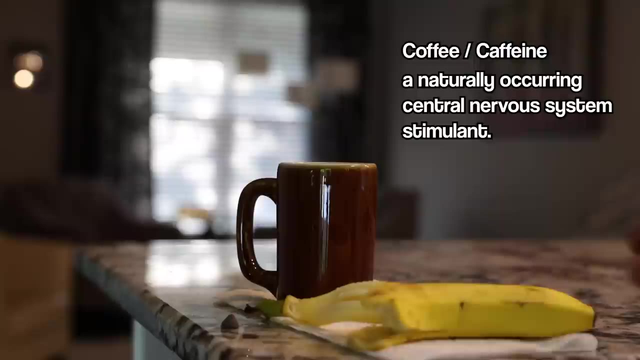 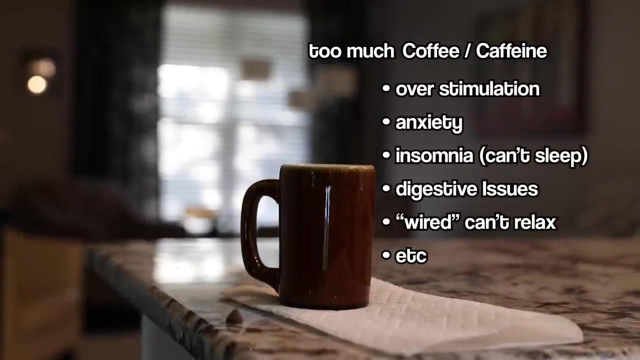 And the caffeine might help me be more relaxed and settled down when I should be there for, leading to better recovery and better sleep and just a better overall rhythm. Now, it should be obvious, but too much of a good thing can turn into a bad thing and coffee or caffeine, while acting as a stimulant on the central nervous system, too much consumption of coffee and or caffeine can result in overall central nervous system fatigue, irritability, insomnia, etc. 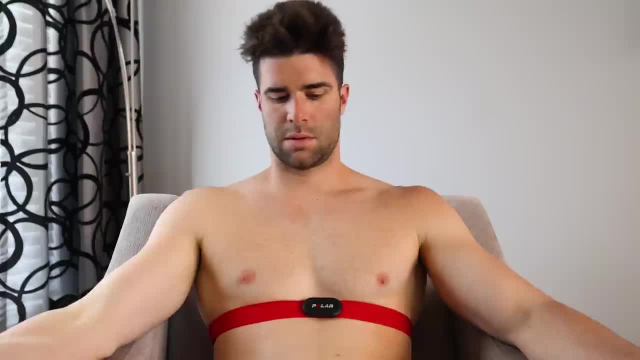 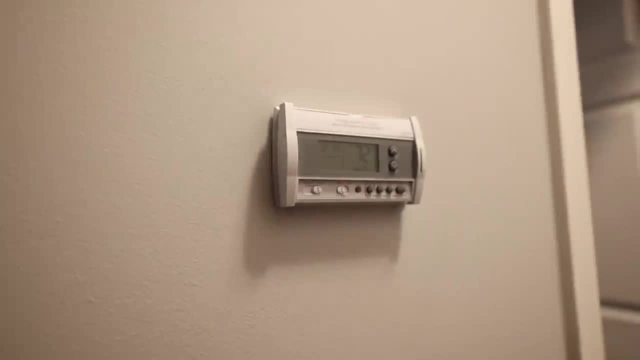 All circling back around To poor HRV. I then implemented the simple breathing routine multiple times throughout the day And then at night I turned the thermostat down because a cooler sleep has been shown to help one settle and maintain sleep better throughout the night. 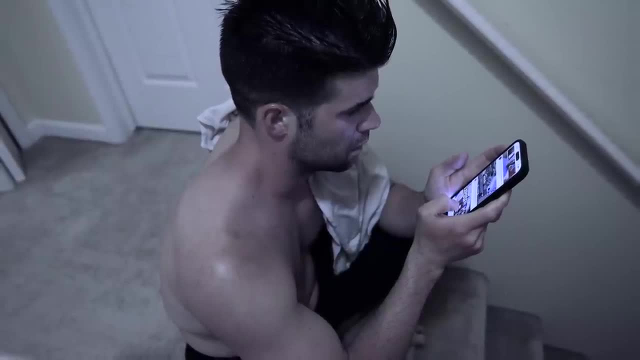 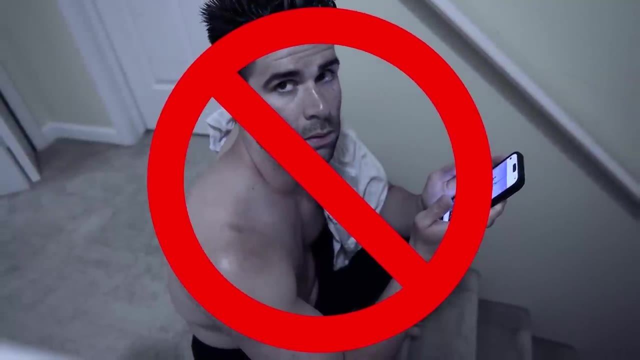 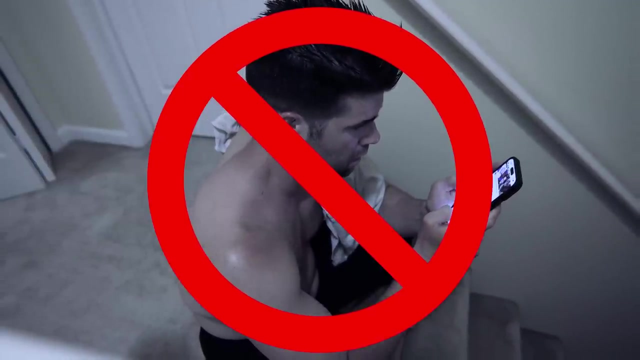 And then something very important I should have already been doing is I got rid of the phone at least one hour before bed. Not only does the blue light from the phone potentially disrupt optimal melatonin production, but also the stimulatory The effects from the phone can have a negative impact on sleep and relaxation. 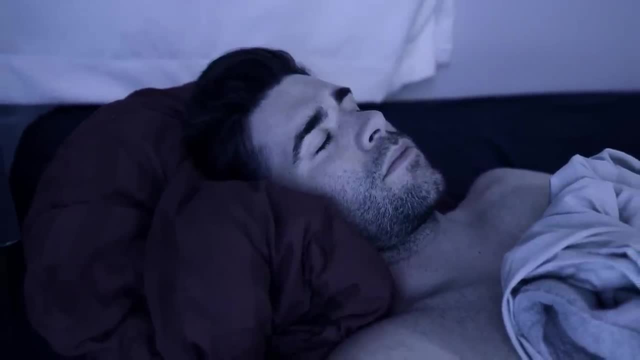 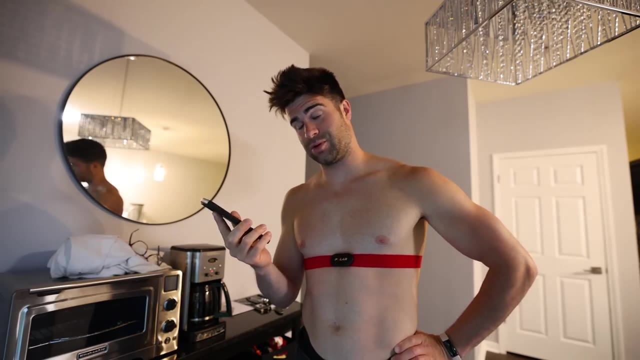 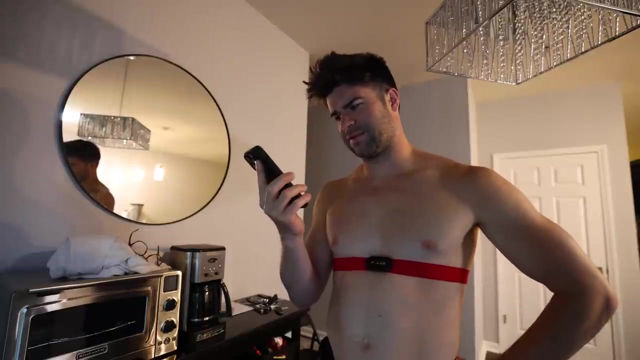 And what do you know? I had a great restful sleep that night and my morning HRV reading on day three was relatively very high, Bro. so my HRV looks like it's way up there at 70 this morning, but it says I'm still very parasympathetic. 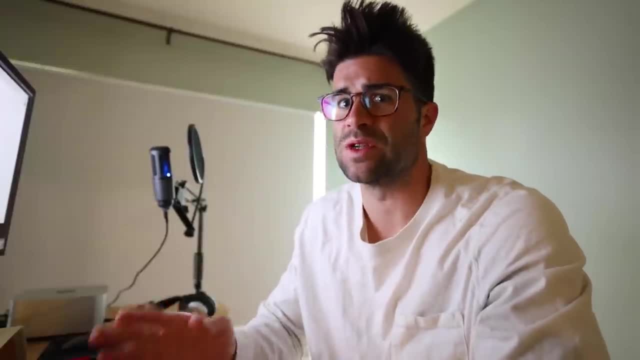 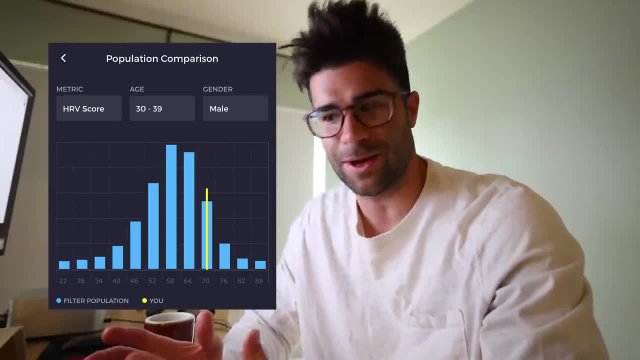 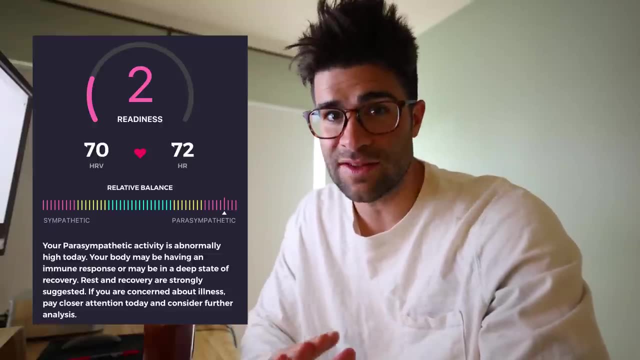 At 70, I'm like dude. am I an elite athlete now? However, according to the app, it said, my morning readiness was off way bad, way too much parasympathetic. However, according to the app, it said, my morning readiness was off way bad, way too much parasympathetic. 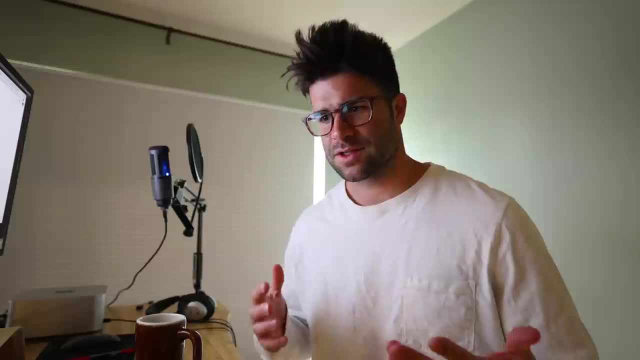 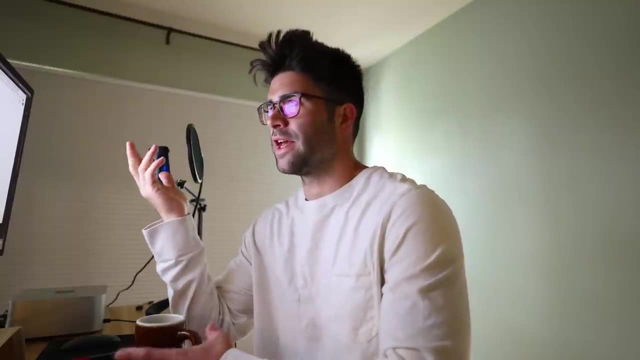 It said I was not ready to tackle the day I might be sick. So I'm like: wait a minute. I have a high HRV score. doesn't that mean I should be more balanced? So I looked into this and according to helpelitehrvcom it says: 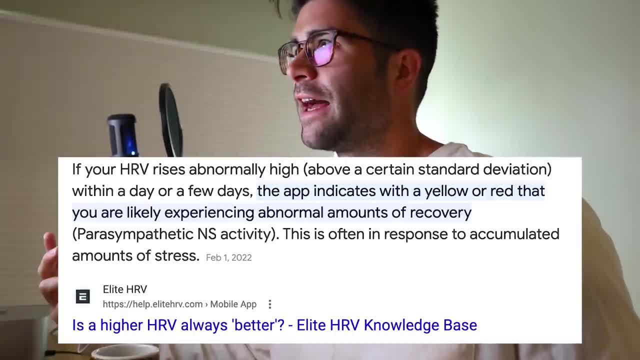 So I looked into this and according to helpelitehrvcom it says: If your HRV rises abnormally high within a day or a few days, the app indicates with a yellow or red that you are likely experiencing abnormal amounts of recovery. 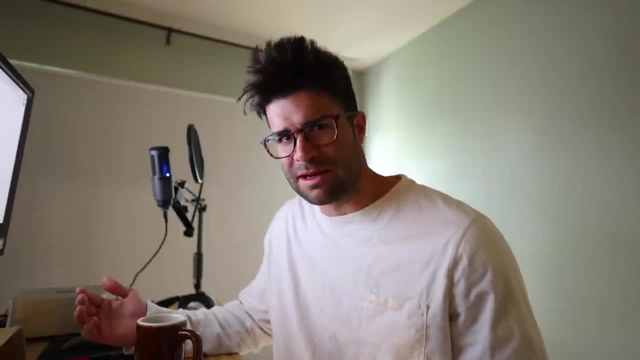 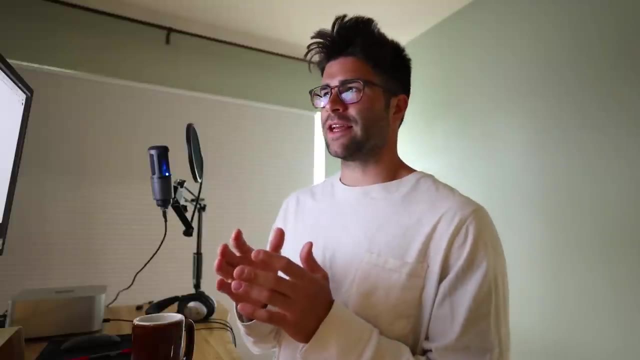 the app indicates with a yellow or red that you are likely experiencing abnormal amounts of recovery. Abnormal amounts of recovery- And they say this- is often in response to accumulated amounts of stress. So what I believe is happening is that I've actually been kind of stressed out chronically for so long. 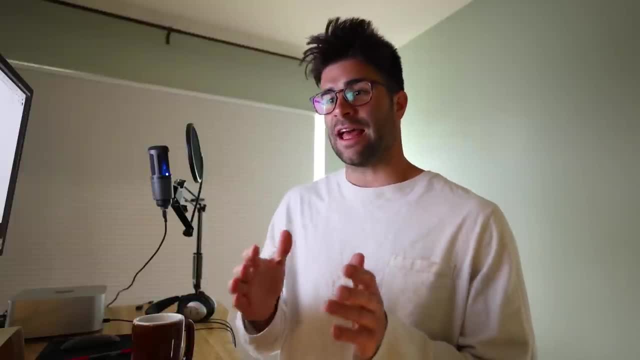 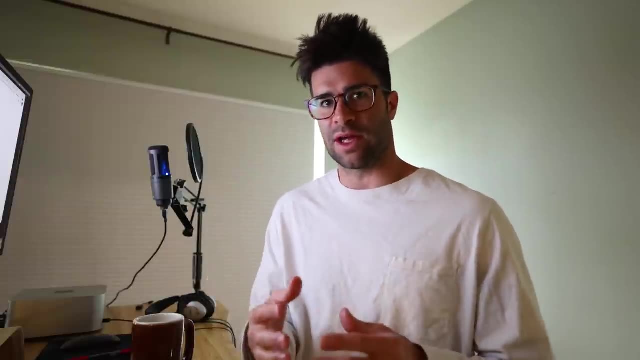 thus leading me to a low HRV score. thus leading me to a low HRV score, getting a decent night's sleep. last night, along with all the breathing exercises and other little adjustments we've been doing, All of a sudden this morning I had a very high HRV reading. 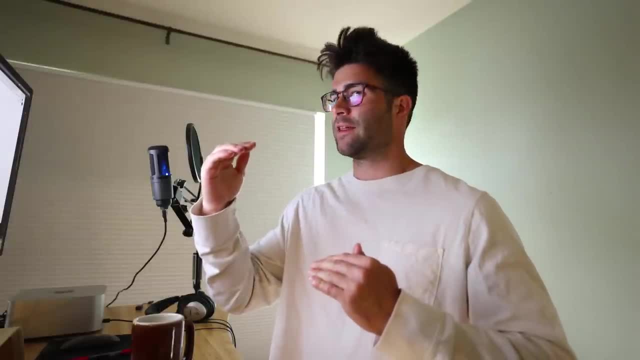 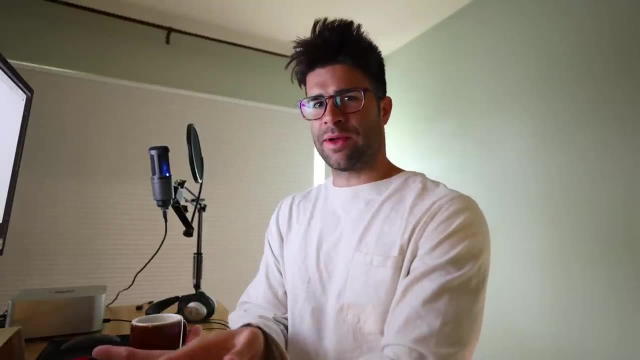 and the app is picking up that crazy variation as Whoa. bro, that's too much, too fast. You must be too parasympathetic. you're not ready for the day. That's how I'm taking it. I could be wrong. it could be picking up some other data. 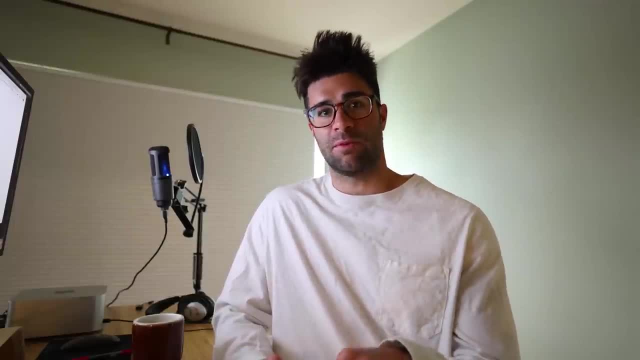 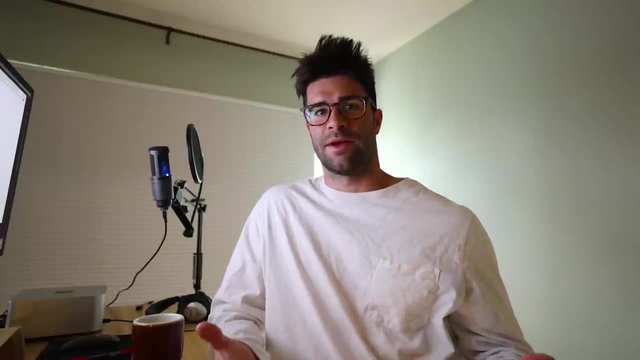 I don't know. I'm gonna continue with the breathing techniques for the day. I'm gonna implement some more things that are said to help the nervous system balance and then I'm gonna continue taking the measurements so we have more data to compare it to. 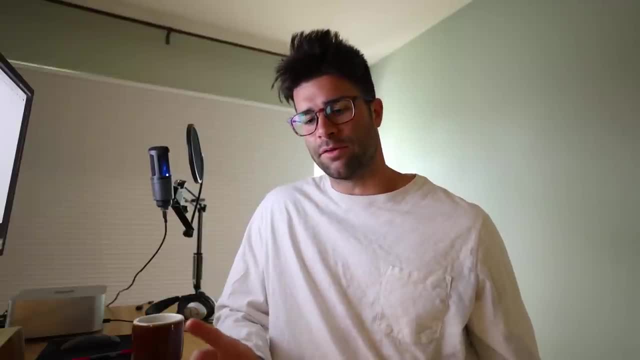 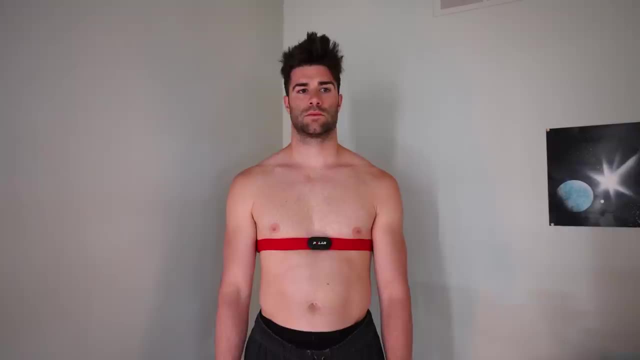 because this just could be an anomaly. I think we're on the up, I think we're improving, but there's still way more work to do. So I continue getting that first thing morning exposure to the sunlight, doing the five and a half second inhale. 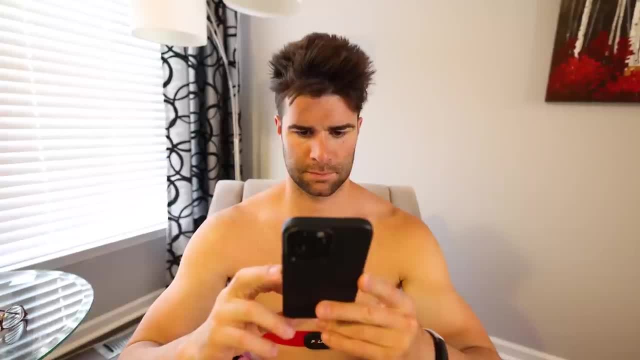 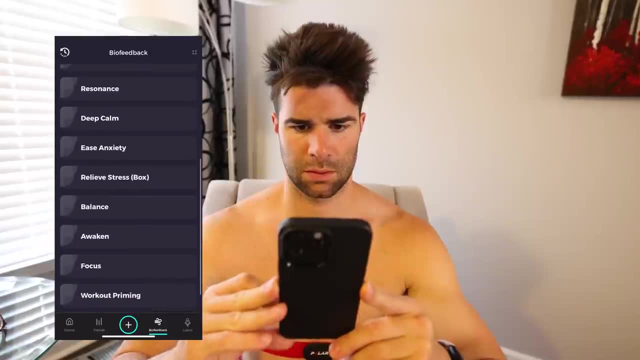 five and a half second exhale breathing routine to help balance. But then later in the day after work I found in the Elite HRV app multiple breathing exercises for different specifications. One of them I found was called workout priming, which consisted of a three second inhale. 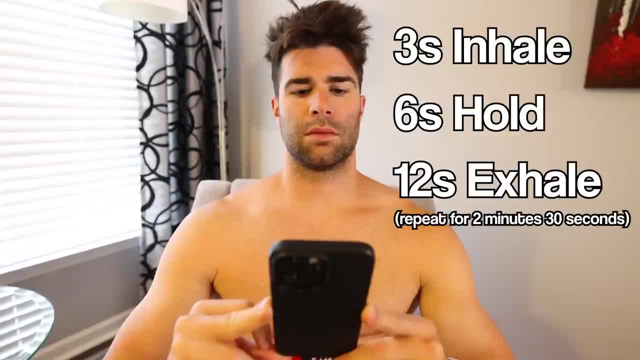 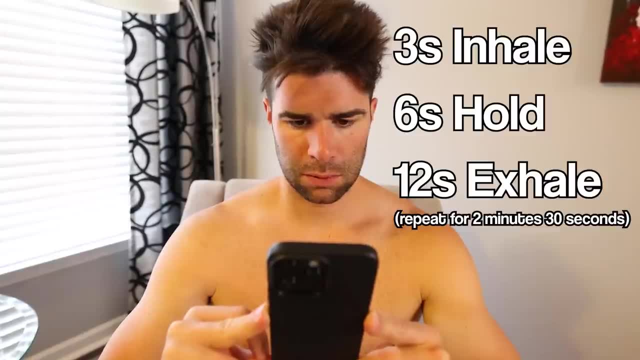 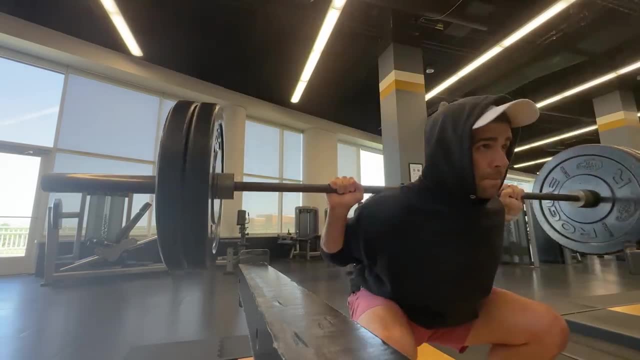 six second breath hold and a 12 second exhale. This, repeated, apparently, would help me prime my heart rate variability and nervous system to perform best in a workout and, to my surprise, it actually felt like my workout went exceptionally smooth. I was focused and explosive, just like I wanted to be. 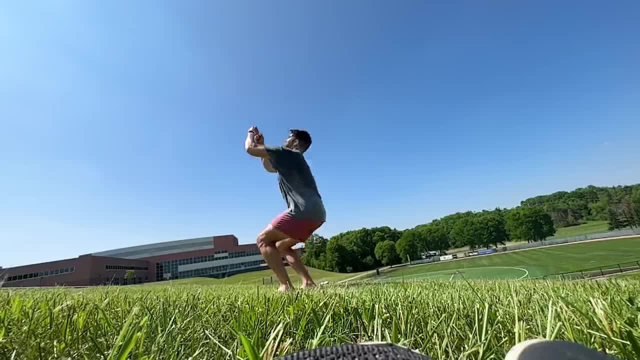 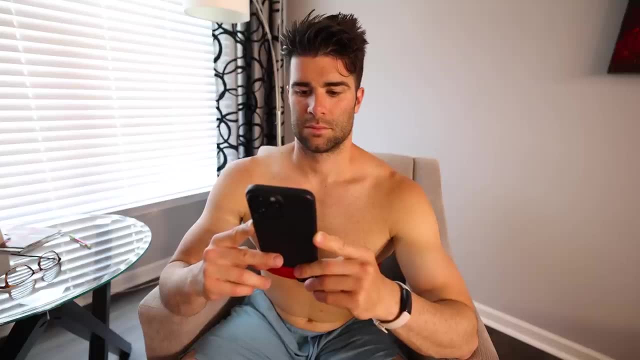 And overall. on top of this, my mental outlook on the entire workout felt abnormally good And positive, if that makes any sense. Liking the result, I went back to the app after the workout and did the post-workout recovery breathing routine. 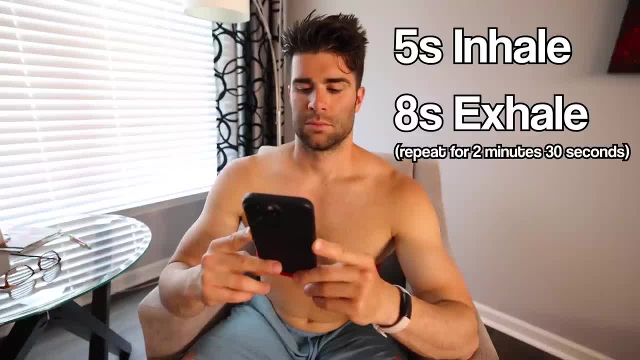 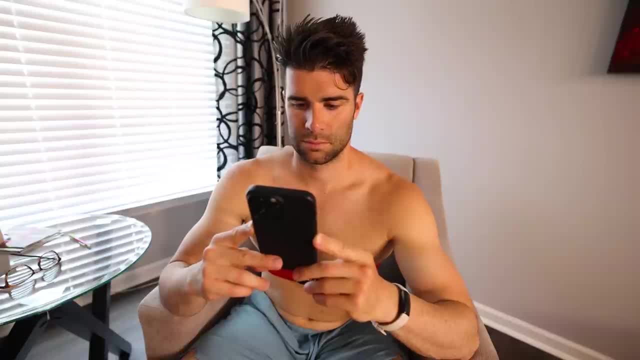 for improved heart rate variability. This consisted of a five second inhale followed by a eight second exhale, And using the app to record my HRV throughout the session. I was happy with the results because overall it seemed like my heart rate variability. 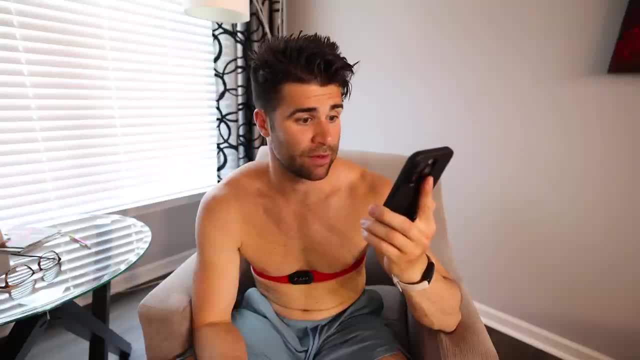 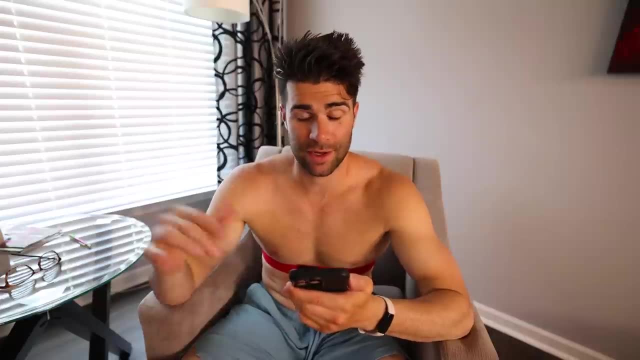 thus readiness and recovery was trending upwards. So my average HRV and my heart rate variability is 64 from that session and my peak HRV was at 71. I'm feeling like we're trending up and I feel like these simple breathing exercises. 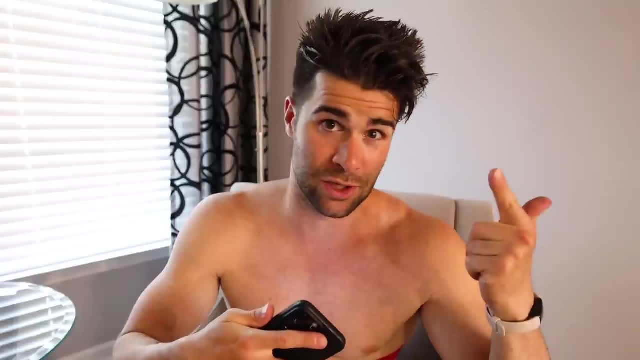 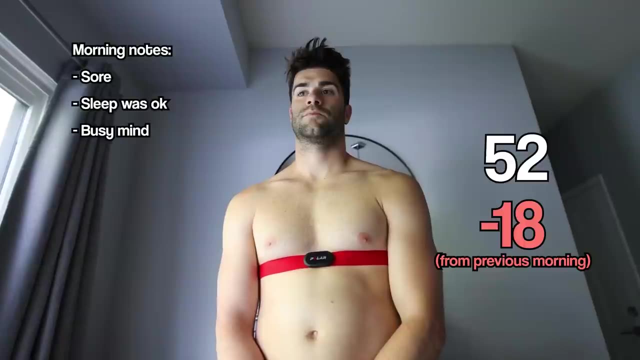 are really helping out, along with the other techniques we're applying. I think we're in the right direction, though Now, unfortunately, the next day, my morning HRV was lower at only 52. And while I slept decently, I felt like it could have been better. 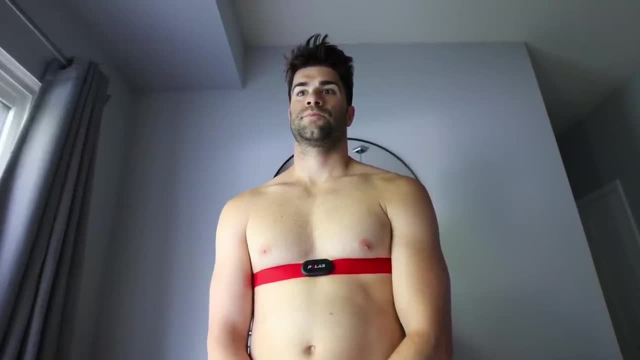 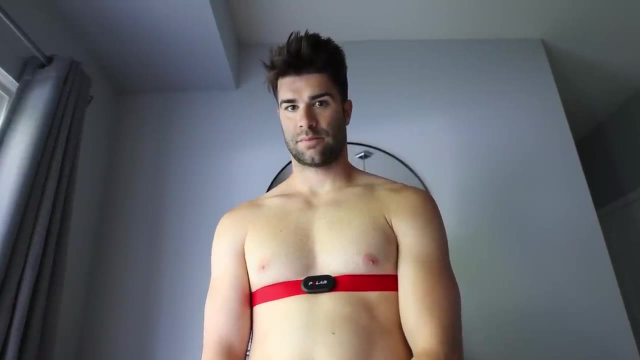 but I also felt like it could have been due to the fact that I was recovering from such an intense, explosive workout from the previous day. Now, something that can better help you understand how your morning HRV readings might be a certain way over time is tracking how you feel in the morning. 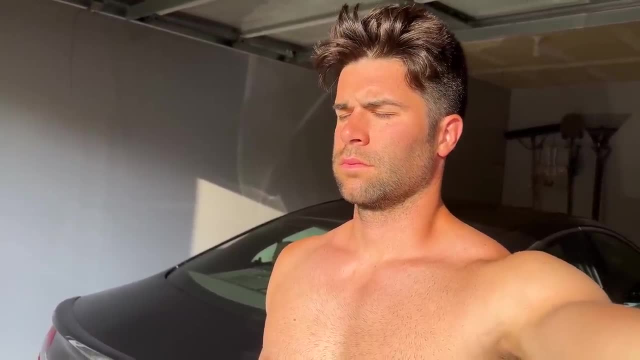 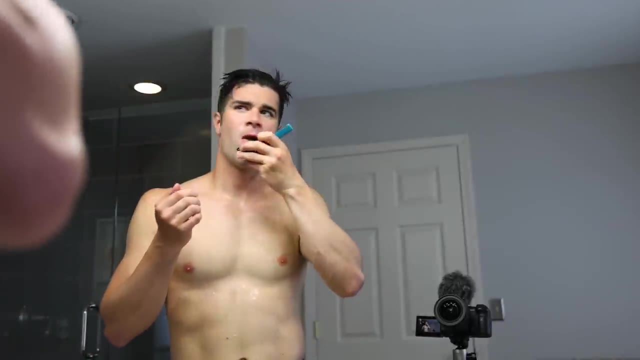 when taking that morning readiness And also maybe tracking patterns or anomalies from the previous day during the next morning's readiness reading. Keeping track will allow you to better make decisions and adjustments to help improve your heart rate variability over time. Now another technique that I've been implementing: 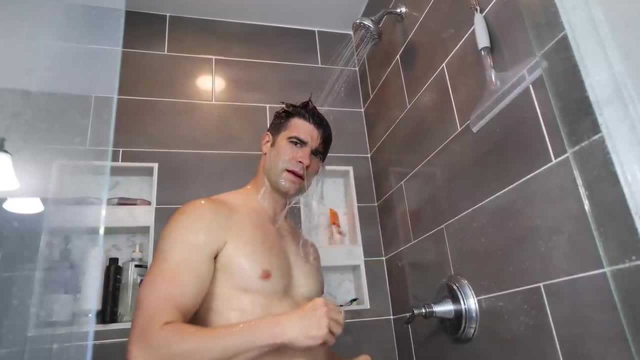 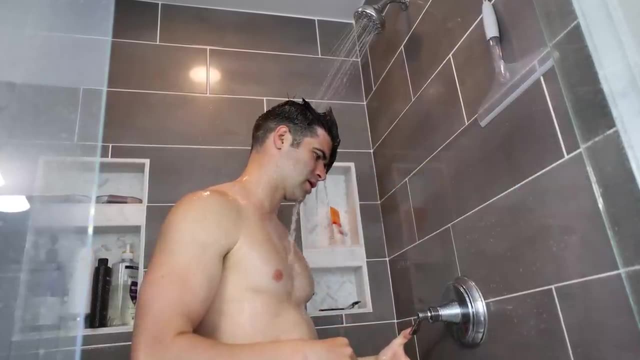 for actually quite a while. that can have a positive impact on heart rate variability is cold water therapy or just taking a cold shower. Now, I don't take my entire shower, but I finish on the cold for about 20 to 30 seconds. 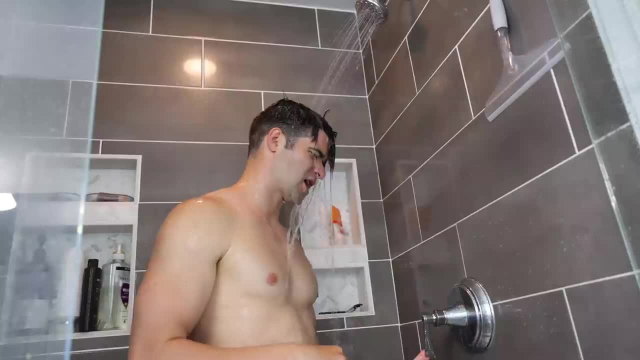 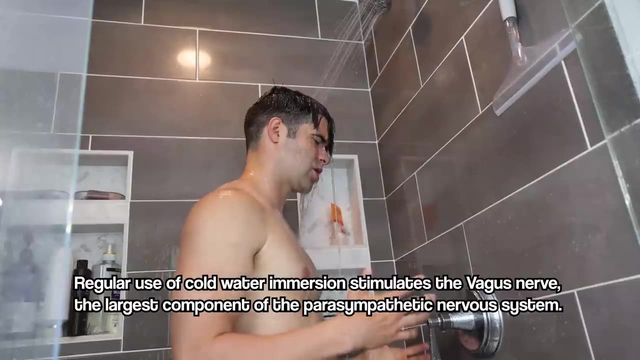 That temporary shock from the cool water can stimulate the vagus nerve which is responsible for controlling most of the parasympathetic nervous system, And from my knowledge this stimulation kind of works like exercise, where occasionally immersing in cold water can help stimulate. 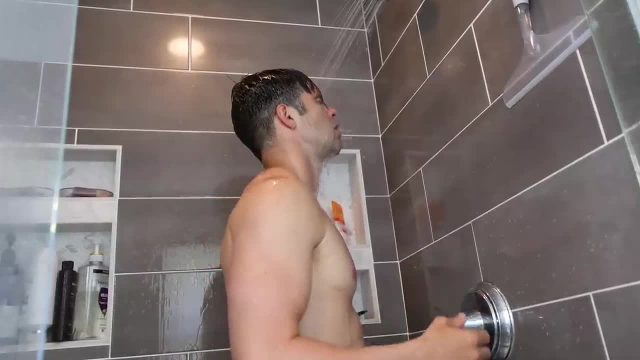 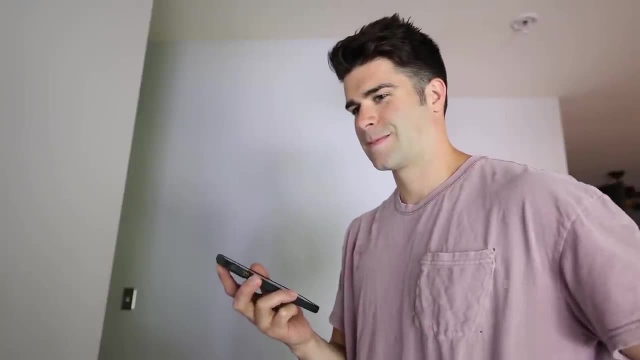 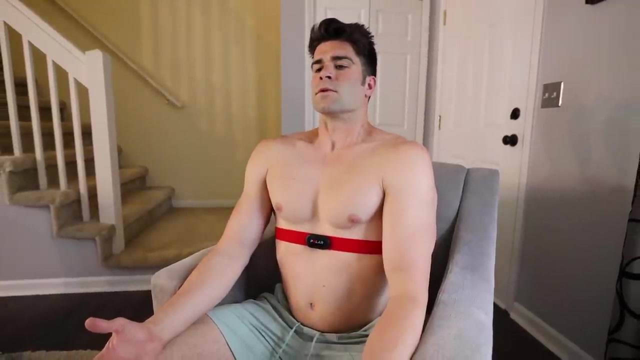 thus strengthen that vagus nerve connection and lead to a more confident response from the autonomous nervous system. Happy birthday to you. So it's my birthday today. yeah, So pretty much just relaxing the rest of the day and trying some more breathing techniques. 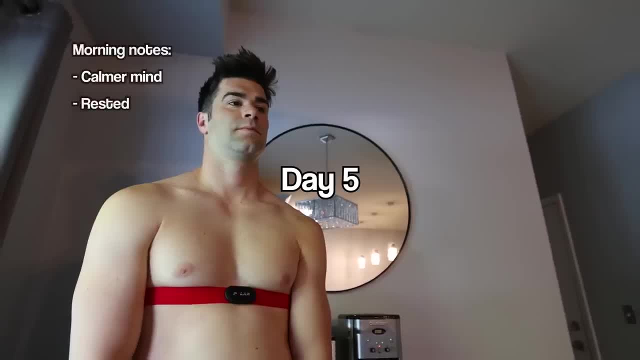 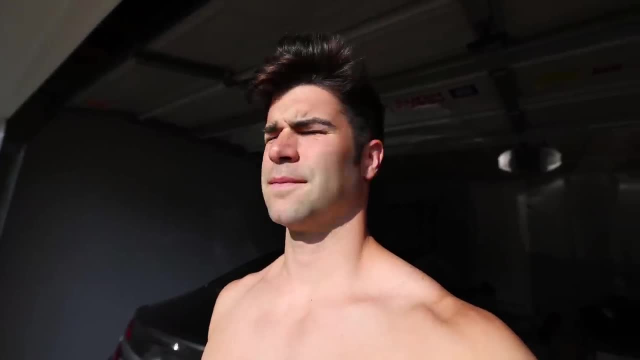 I found myself feeling peaceful and balanced by the end of the day, And then on the next morning my heart rate variability was up to a 57. So overall, the cluster of these last three days was trending up, which was good. I continued implementing these various 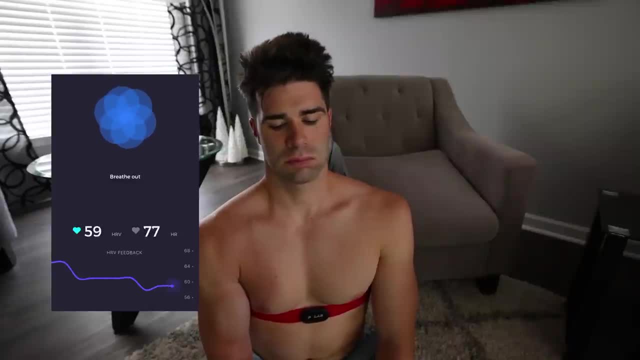 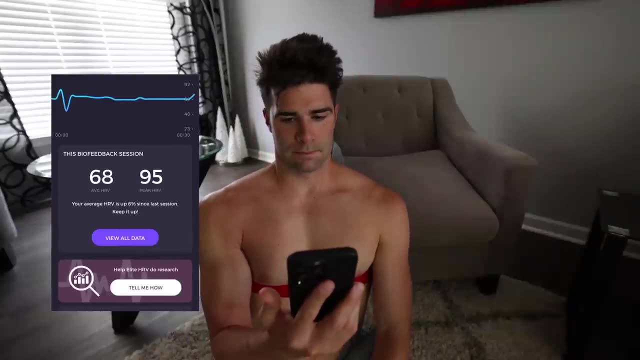 around three minute breathing routines based on how I felt throughout the day: whether I was about to go into a workout, trying to recover from a workout, awaken, relax, et cetera. Everything was looking good, But that is all until later in the day. 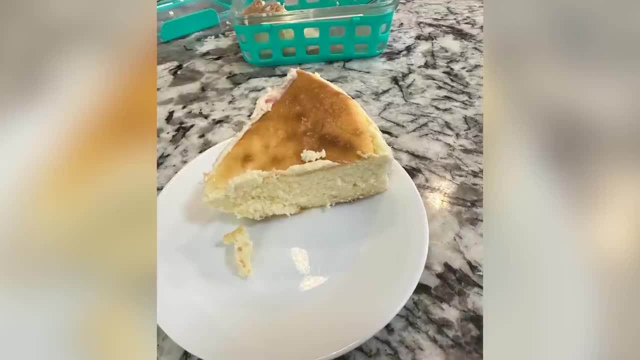 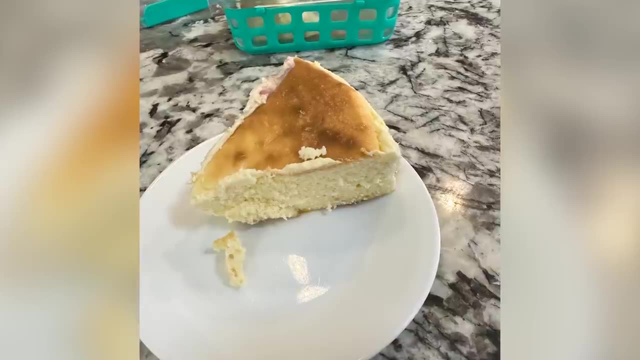 I ended up indulging on way too many leftovers from my birthday party celebration, But, let's just say, consisted of a lot of cheesecake and leftover carryout food that I'm not used to and food that may not be considered too healthy. Oh man, oh. 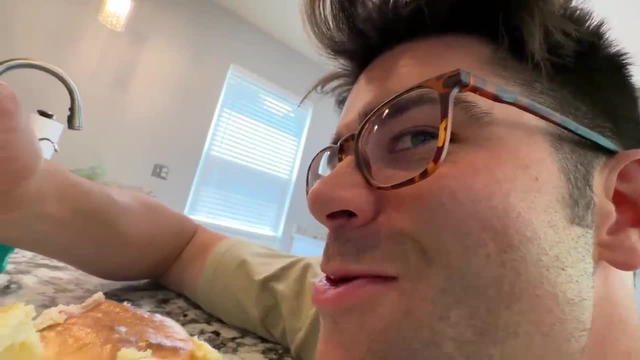 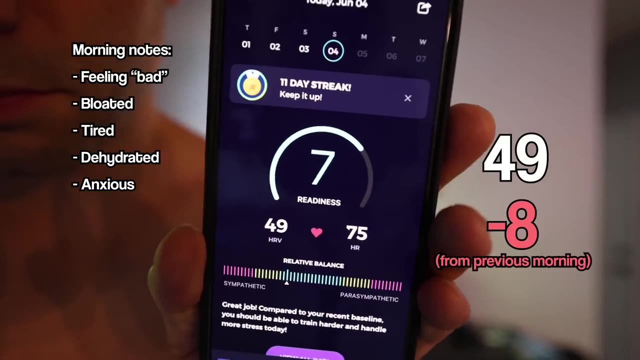 I shouldn't be doing this, but it's my birthday And what I believed was because of just the diet change this day, my next morning's HRV reading was back in the 40s, So diet really affects HRV. Holy smokes. 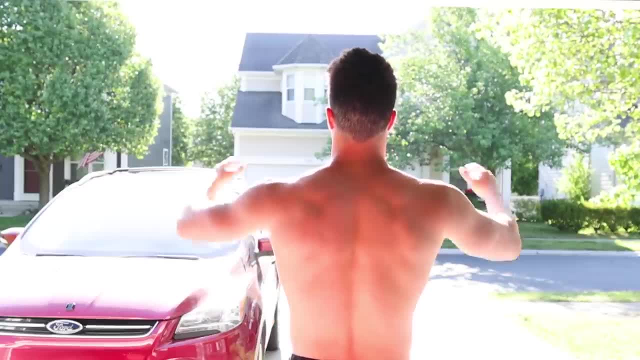 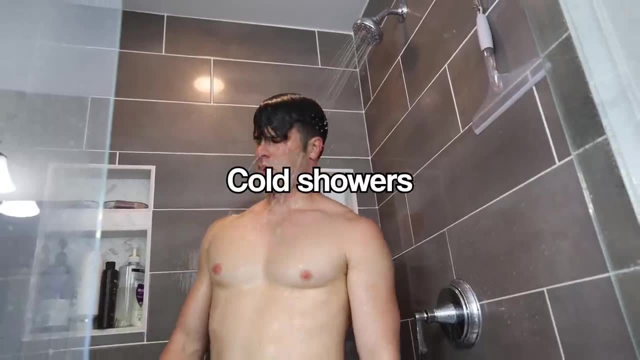 But I managed to stay positive and just get back on track, implementing the various techniques I was learning throughout this experiment, focusing on that morning: sunlight, focused breathing, cold therapy, eating healthy, limiting light exposure before bedtime, especially no phone, and just by that already by the next morning, 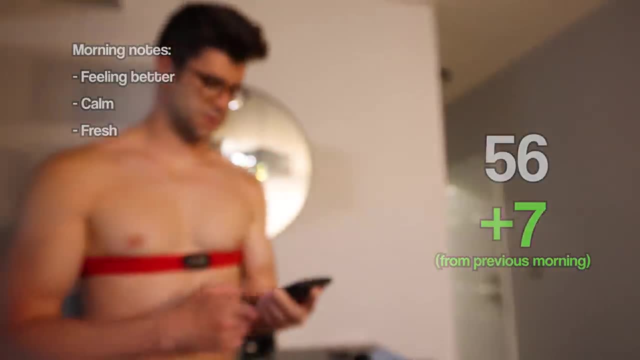 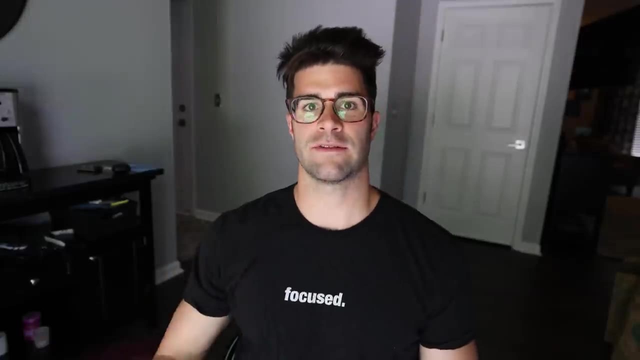 my HRV was significantly improved, Coming back to normal there. so that's about it. What's up Home Slice? So this has been an absolute eye-opening experiment, If you think about heart rate variability as we looked at it throughout this video. 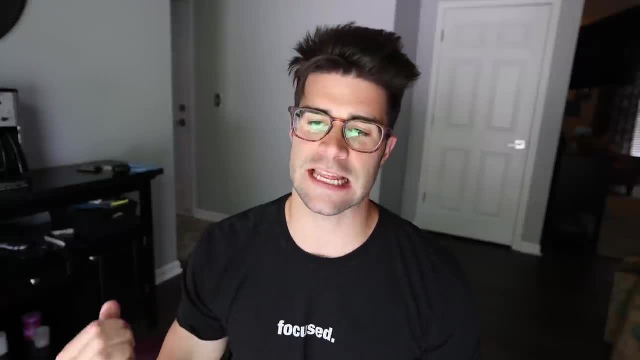 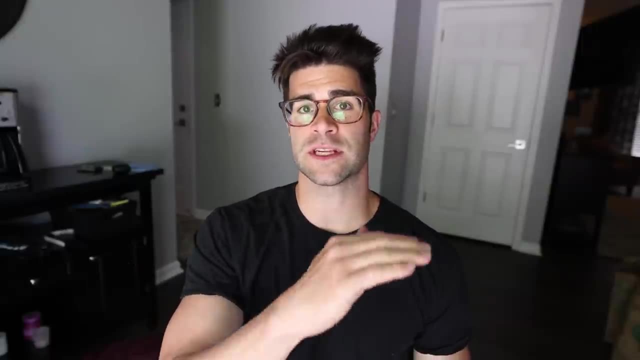 and how it can be applied. and why it's so important is because it is this reading that is so correlated with overall health, wellness, performance, et cetera, that we can use it, when tracked consistently, to determine what might affect us particularly. 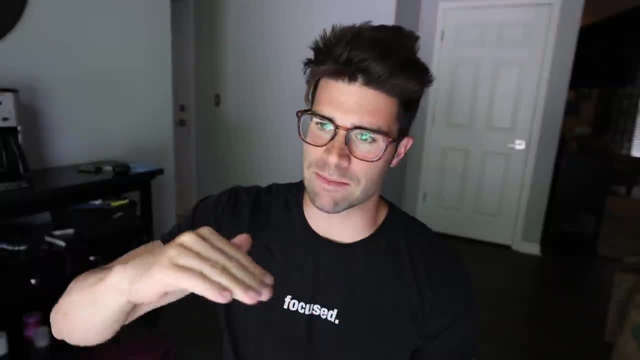 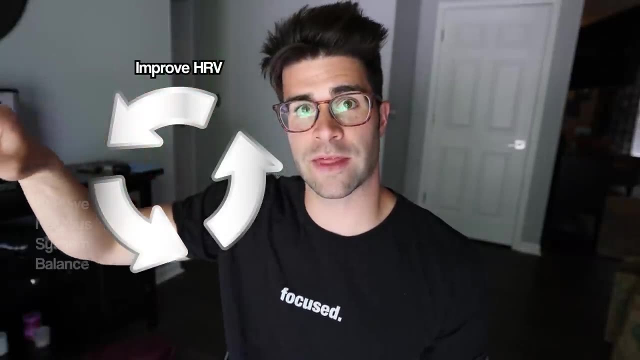 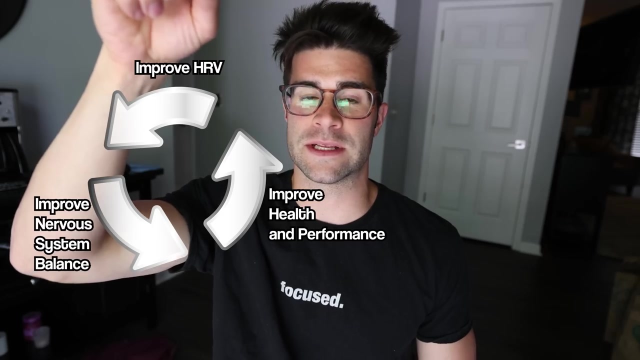 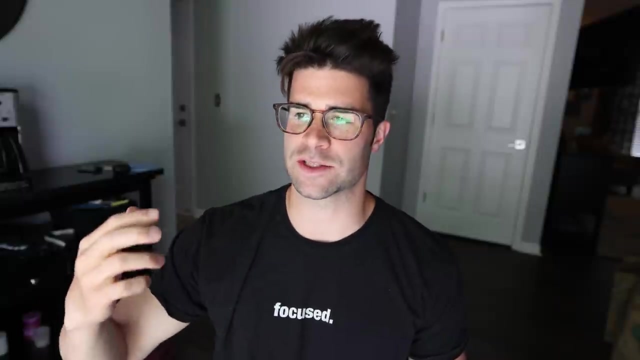 вр positively or negatively and how we can possibly trend up, and thus trending up hrv will, in return, full circle, help improve that balance, and that better balanced, healthy response will therefore improve health, improve athletic performance, improve mental state, well-being, etc. it's this positive circle and that right there should be obvious why it's so important for elite athletes. 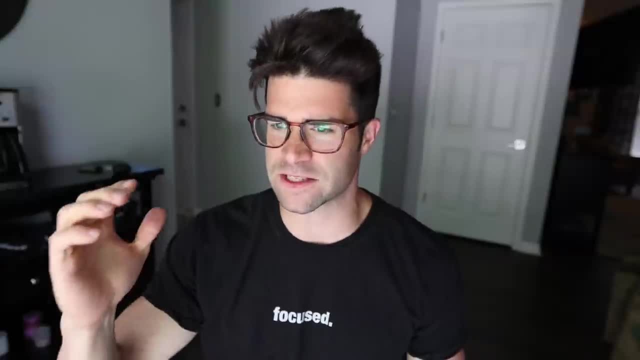 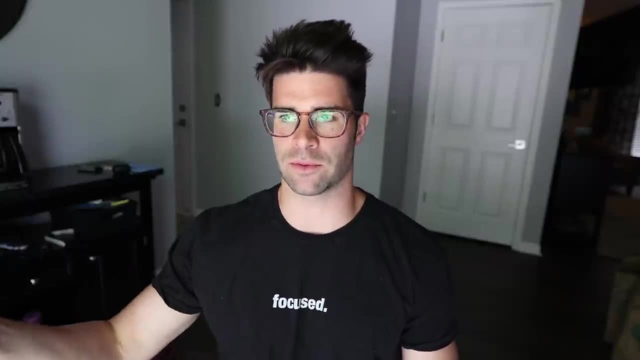 coaches, people who want to improve their mental, cognitive, physical states. trying to just be a biohacker, you know what i'm saying? i mean, it's non-invasive. it gives you these readings and you can just watch it either improve or degrade and make adjustments over time. now, with that being, 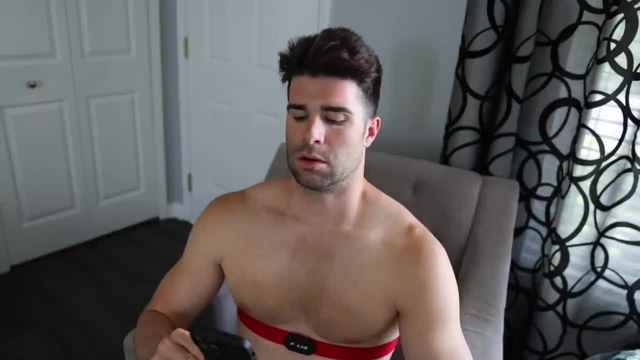 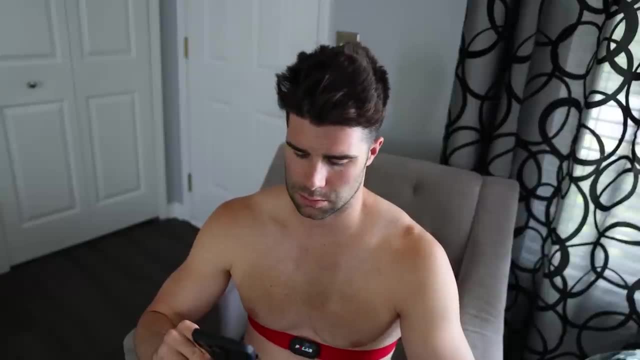 said, we saw in this experiment that by doing a simple breathing routine of just that: five and a half second inhale, five and a half second exhale, approximately six breaths a minute, can instantly balance the autotomic nervous system, leading to a balanced, improved hrv reading. so this is just a great, simple tool to use. however, based on my research- and what just makes sense is regarding overall heart rate variability, i found it important to measure it consistently in the morning because that's kind of showing like where we're starting our day off at, and i saw in this experiment after taking those. 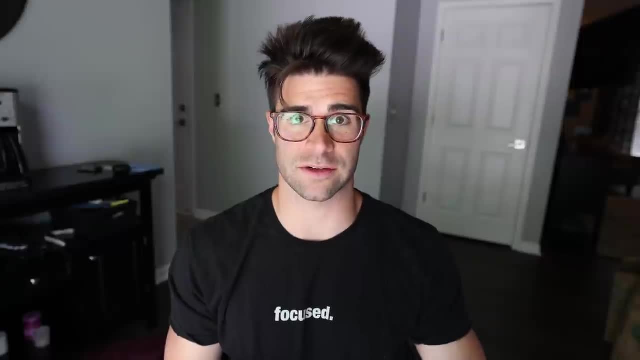 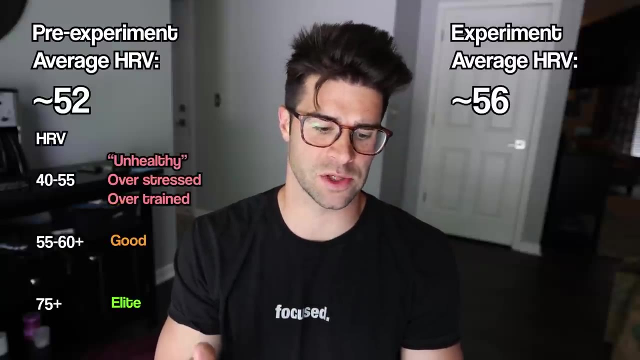 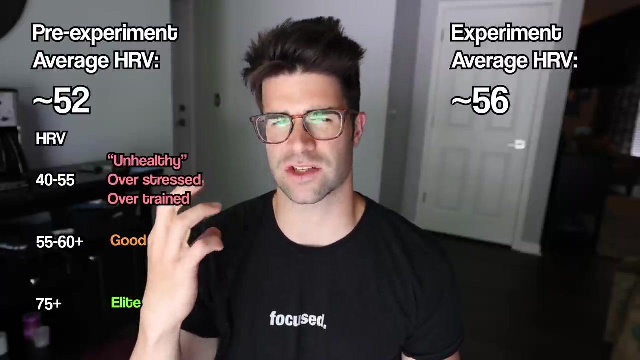 first five readings before starting any of these exercises, that my average hrv was kind of low. in fact, it was actually in the what i found to be the unhealthy range, which apparently is between about 40 and 55, and i think this was due to just having too much like chronic stress built up in my mind. 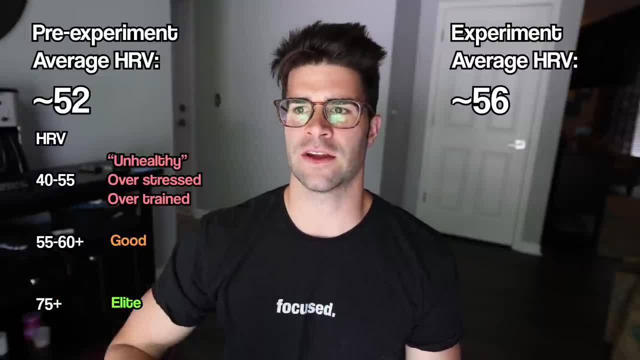 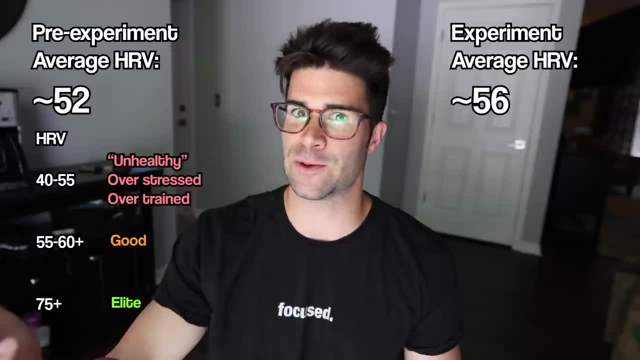 every single day and i really wasn't taking the time to relax, to just breathe, and i wasn't focusing on good sleep. i was looking at my phone before bed. i know it's stupid, i knew it was wrong, but i was doing it. i wasn't balanced. i didn't feel balanced now. on those days i had better hrv. 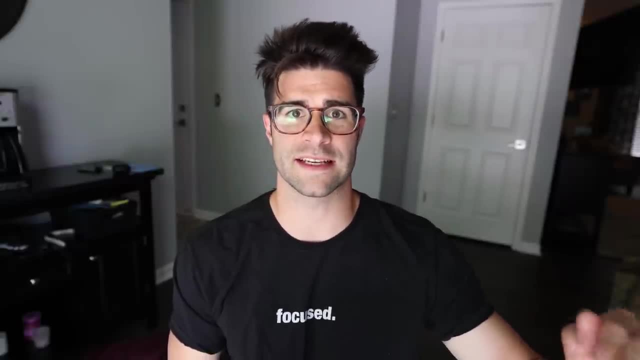 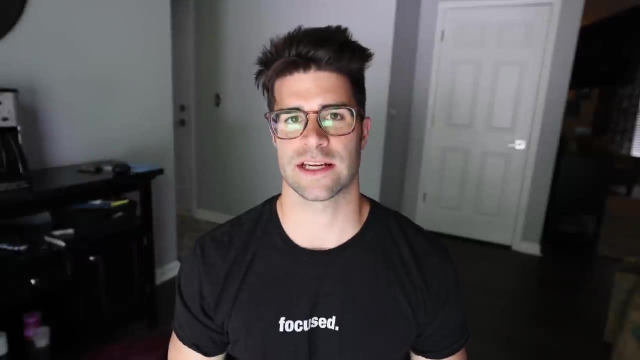 readings in the morning, i felt like my overall day went significantly smoother- from my work to my workouts to just my overall mental state- and i was able to do a lot of things that i wanted to do. state and, based on what i experienced, i would like to further continue to try and improve this. 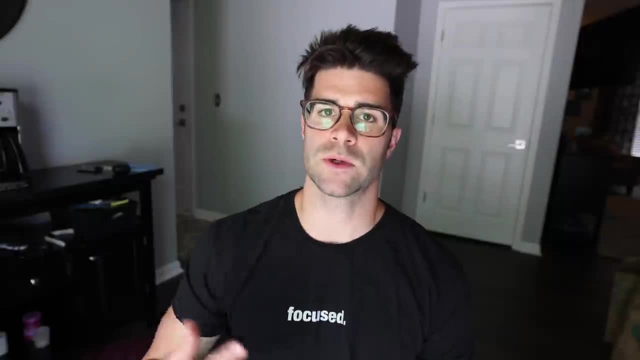 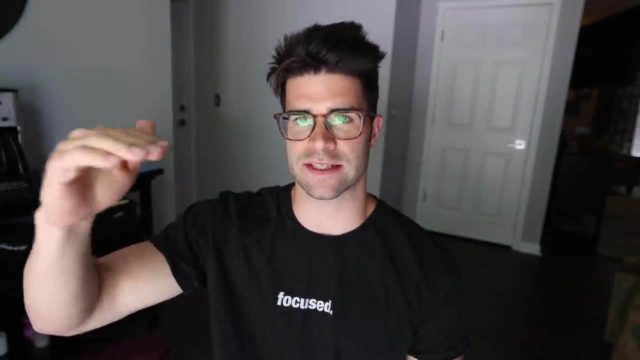 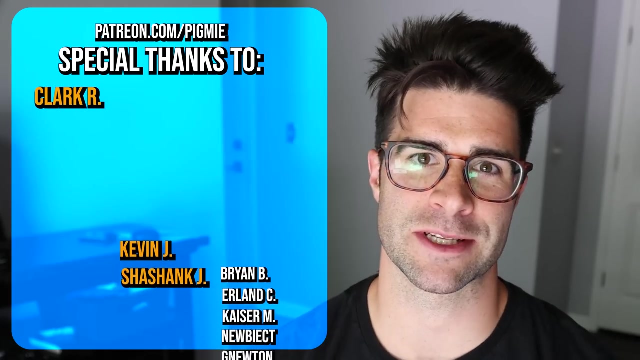 reading by improving my overall health. so what would be most important to me going forward is to continue taking these morning measurements and trying to get that morning measurement on average consistently higher than it was for, like the previous week, let's say. hope you all enjoy this video. don't forget to subscribe. stay tuned. more experiments coming out, peace, i will see you. 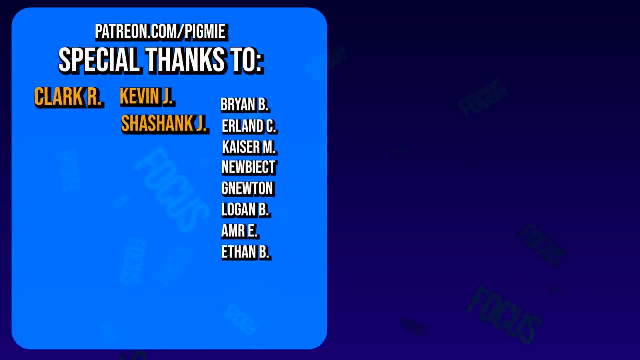 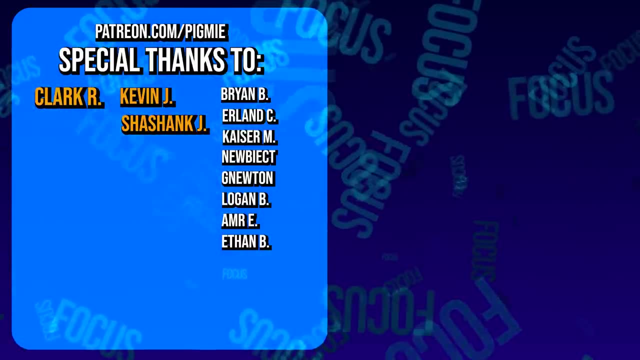 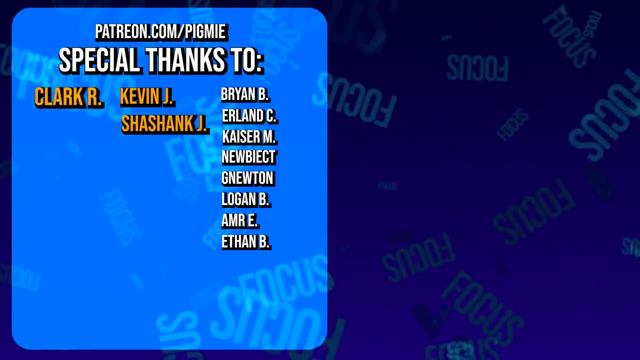 in the next video. you.